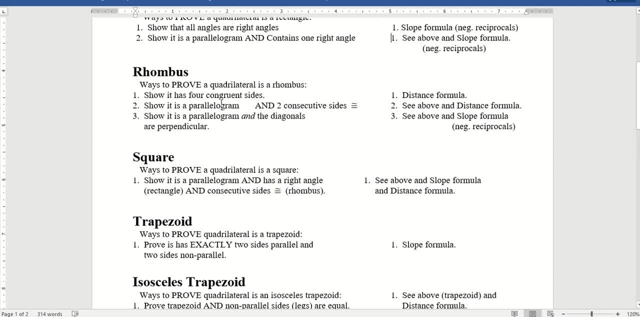 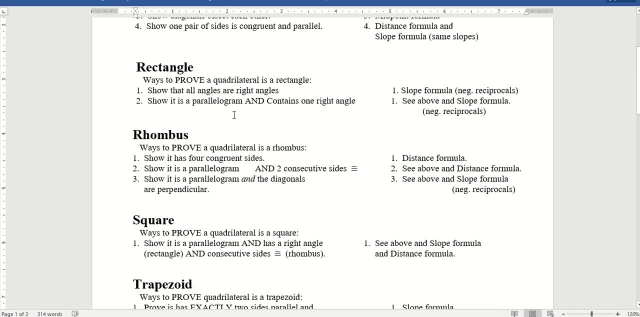 angles and then we'll talk about that. then we get there. so we're going to focus today just on the rectangle here, right, okay? so we want to either get all the angles to be 90 degrees or we want to show it's a parallelogram and then has one right angle. but the easiest way to do this, the way that we're 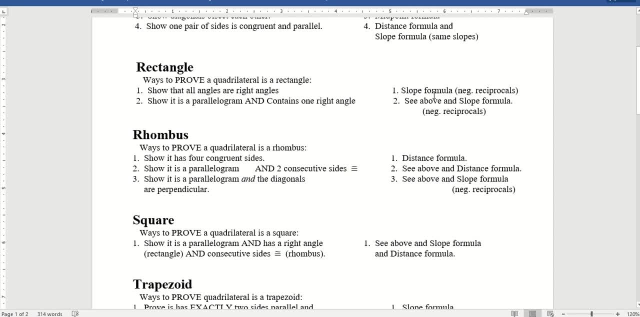 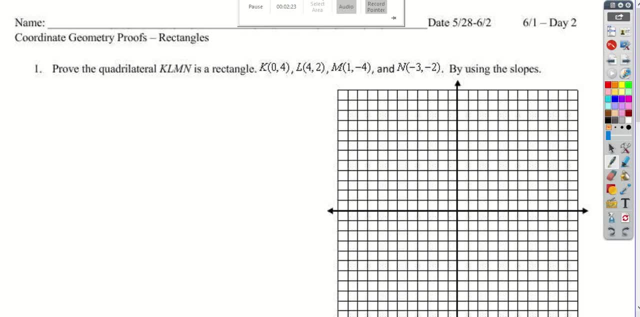 going to focus on here, okay, is that we are going to use the slope formula. all right, that's the big thing here. okay? so let's go back. so we're going to go ahead and graph our shape first. so go ahead and do that for yourself. and so here's k l m n, and so we're going to use the slope formula here. okay, so we're. 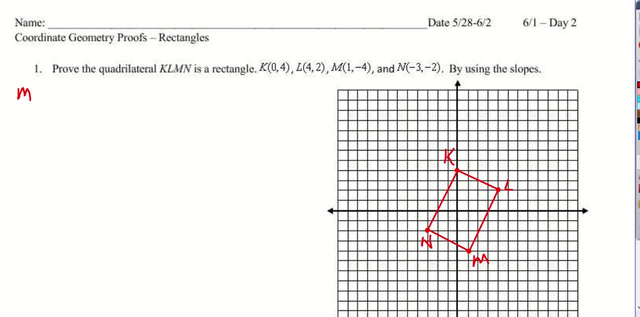 going to do the slope, so we're going to do m to represent slope, and then we're going to put k l next to it because we're doing this slope of line segment k l. remember we're going to do four slopes, so we want to keep track of them. okay, remember the rule or the formula is y2 minus y1 over x2. 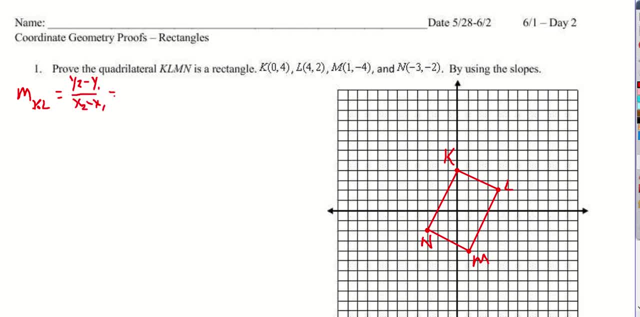 minus x1. now i'm using the how the points are written here. k is first, l is second, to do x1, y1, x2, y2, so it says y2. we're going to go to the second point, which is l, that's 2 minus y1, which is 4. 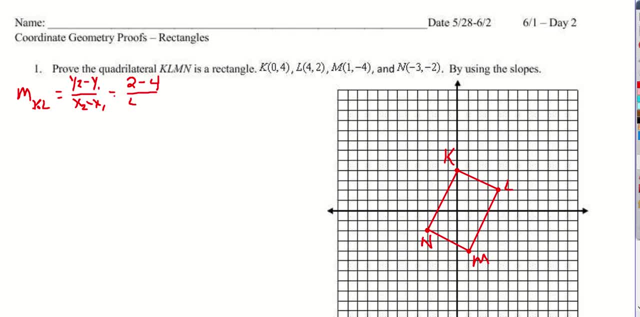 from k and x2 from l is 4 minus k, which is 0. now the big thing is is you just want to make sure that these points for l are stacked over each other. so the 2 is on top, the 4 is on the bottom. 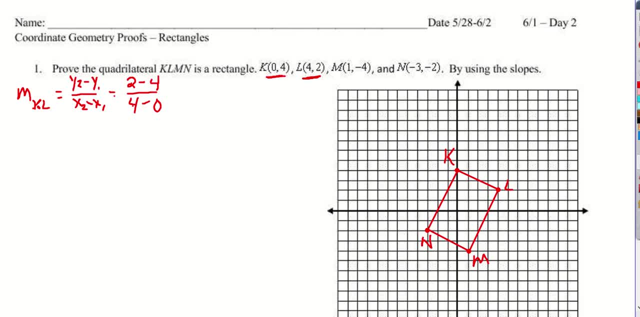 same thing for k is that they're stacked on top of each other. so technically, if i put the uh, the 2 and the 4, like if that was my y2, y1, that's fine as long as you're consistent with putting what points on top of what here. and then i'm going to subtract. so 2 minus 4 is negative. 2, 4 minus 0 is. 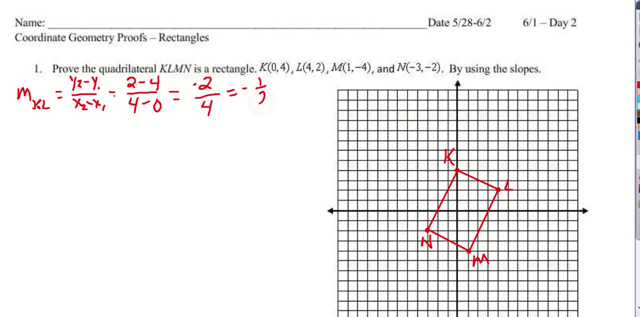 4 and so we're going to reduce down and get a slope of negative one half, and i always want to reduce because the numbers could be different. i could be like negative 4 over 8, but i want to know that it gets the same uh fraction in the end here, that we're equal to the same thing all. 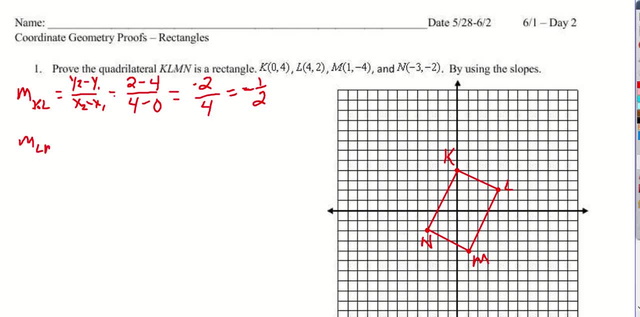 right, so the next slope is going to be l- m. those are the next two points, and so, once again, i'm not going to write down the formula again, but we're doing y2 minus y1. so i'm going to m. y2 is negative, 4 minus y1, which is now 2 over, and then for m it's 1, that's the x coordinate. l is 4, so 1 minus 4. 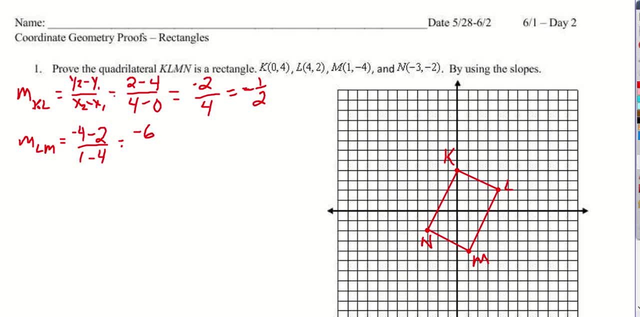 minus 4 is negative. 6 or negative. 4 minus 2, 1 minus 4 is negative. 3 and a negative over a negative becomes a positive, and so this is just positive. 2, which is also 2 over 1, and as you can, 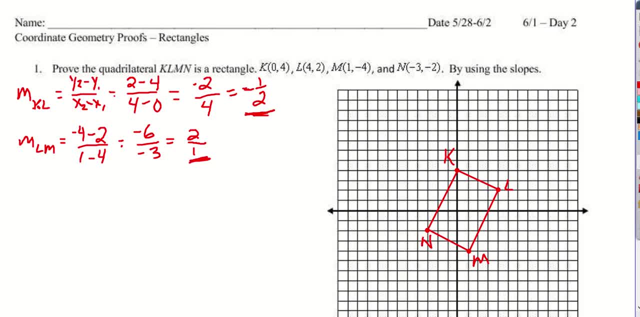 see we have negative one half and positive 2, so we do have opposite reciprocals. these are: change the sign, flip the fraction. these are negative reciprocals, which is what we're looking for. so that's good, okay, slope. the next one is going to be m? n, so we're going to go. second, same thing: y2 is negative, 2 minus y1, which is: 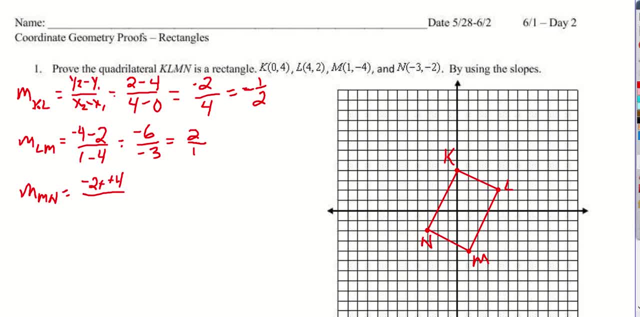 negative 4, so that double negative becomes a positive, and then it's negative 3 for n minus negative 4 again. that's a double negative negative. 2 plus 4 is 2, negative 3 plus 4 is 1, and we get 2 over 1 again. okay. 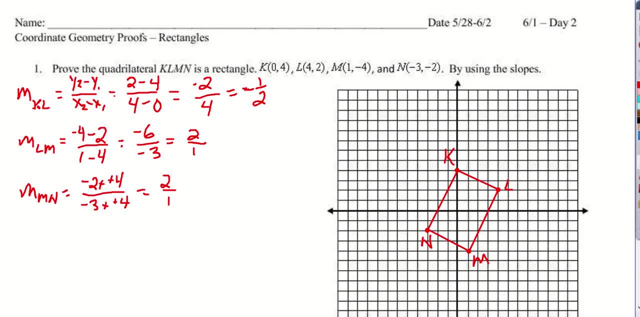 um, double checking caught the problem. do you see the problem? i see the problem now. that's why i wasn't looked. now i'm here's how i'm catching my air. kl is over here and m n is over here, so these two sides should be parallel and i got different sides, so i'm going to go second same thing and i'm going to go. 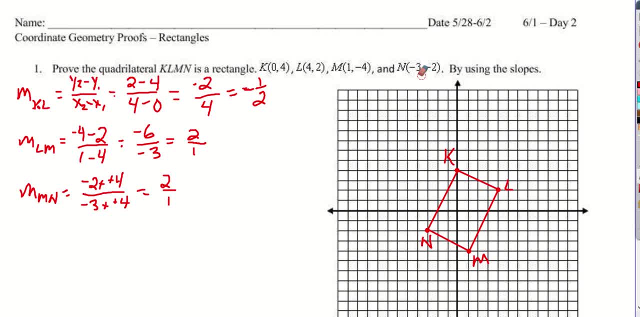 negative 3, okay, negative 3, right. and then negative 3: 1 minus negative 3 over here, plus negative 3 plus negative 3 over here. so we got almost all right. we got everything. our zero points have two six points, one negative three each one right. and now we're going to go into. 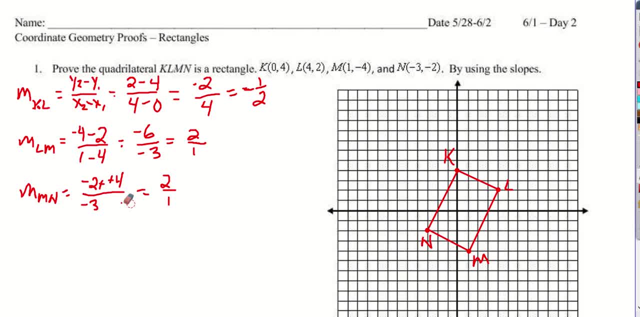 negative 3 if you could just go back to the first one of your ziezee. so this is the first one right here and then i'm going to uh once i get from here. so because they needed it and you're getting between this way in slightly where we went to um, so you 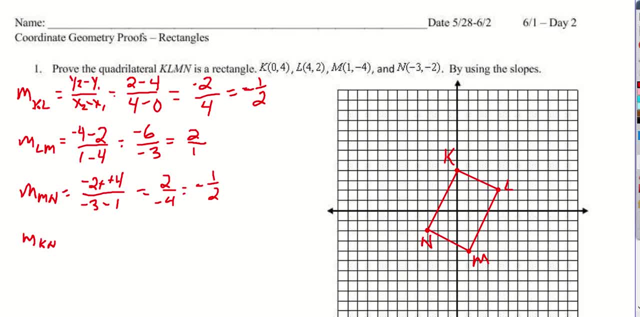 point. so kn is the other line. Okay, so we're gonna go from n, that's y2 is negative 2 minus k, which is 4, over n, which is negative 3 minus k, which is 0.. Okay, now, remember, we already know that this should be like negative 6 over. 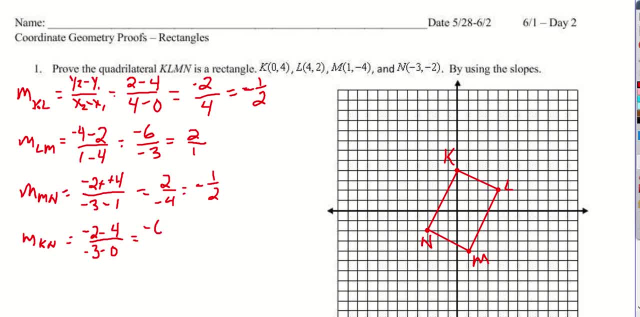 negative 3 and 2 over 1. so negative 2 minus 4 is negative 6. negative 3 minus 0 is negative 3, and that becomes 2 over 1.. Alright, so just cleaning up this: equal sign here equals 2 over 1.. Alright, so now we have enough to say that this 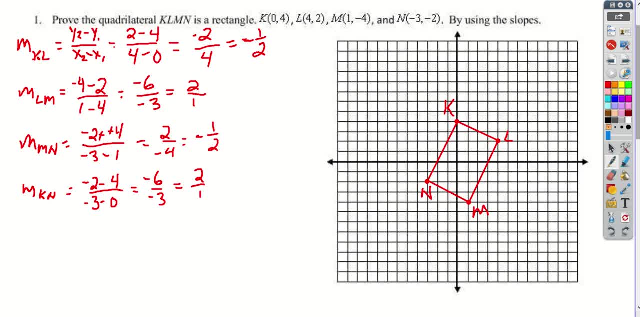 thing's a parallelogram, right, We have opposite sides parallel because we have the slopes are equal and we also have that each of these slopes, right, are opposite reciprocals to one another, so they all are gonna form right angles. Okay, So we want to go ahead and make a quick statement and then our summary. 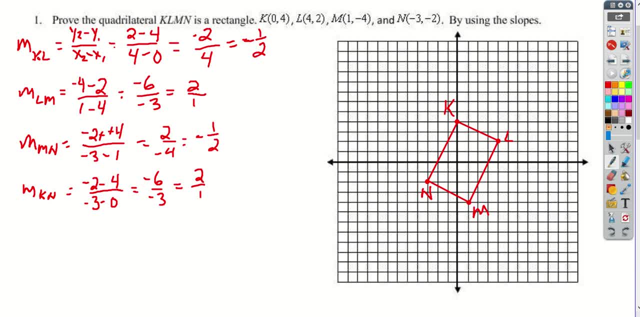 statement: Okay, and so we're gonna say that two things we can do. We're gonna do the, we're gonna do straight rectangle. We're gonna say: kl perpendicular to lm, comma, lm is perpendicular to mn- comma, mn is perpendicular to kn- comma and kn is. 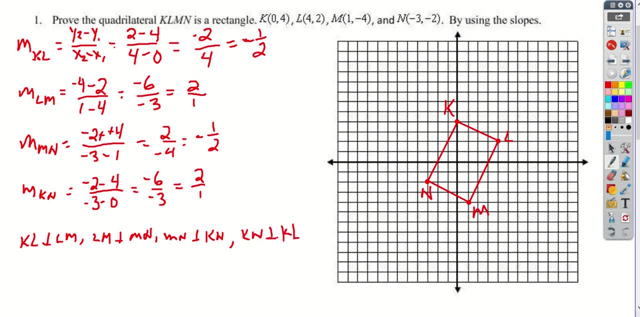 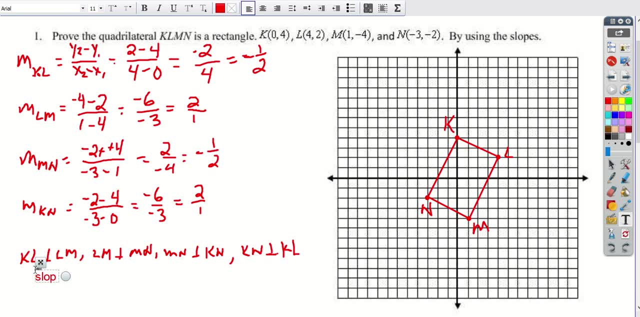 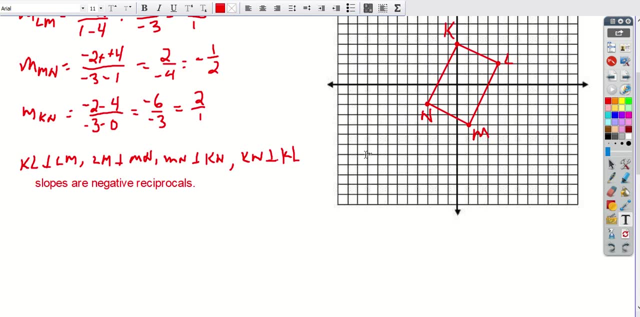 perpendicular to kl. This is one way to do this, Okay, and so what we're gonna do is we're gonna say right underneath why this is true, and we're gonna say: slopes are negative reciprocals, alright. and then we're gonna write our summary statement at the 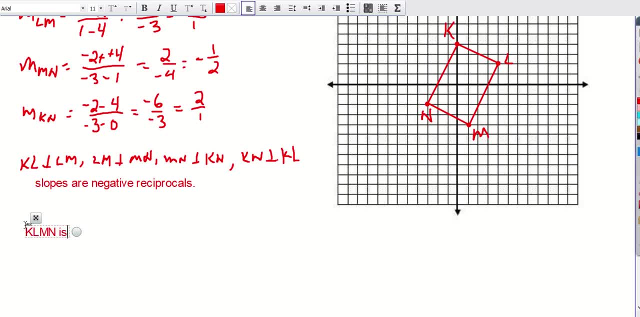 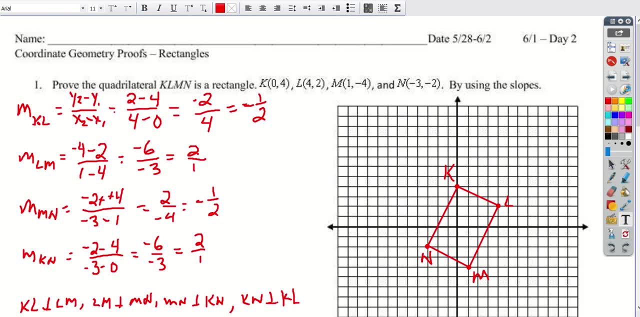 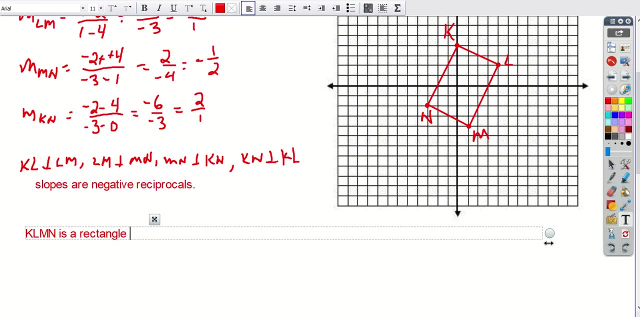 end, We're gonna say that klmn is a- what's the name of our shape, by the way? Where'd it go? Yeah, it is Alright, couldn't see it. there is a rectangle, since it has four right angles, okay. 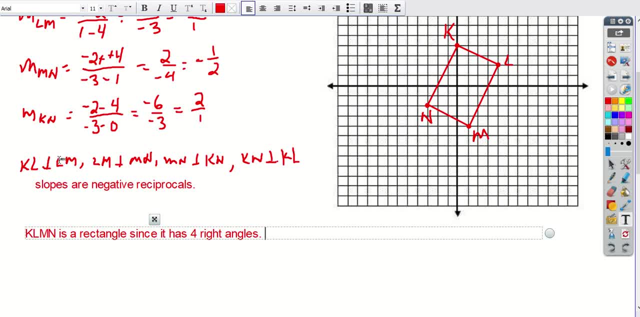 Now, the other way we could have done this is to say that it's a parallelogram, because the opposite sides are parallel with the same slope and it has right angles, since the opposite sides have consecutive sides, have opposite reciprocal slopes. I like doing it this: 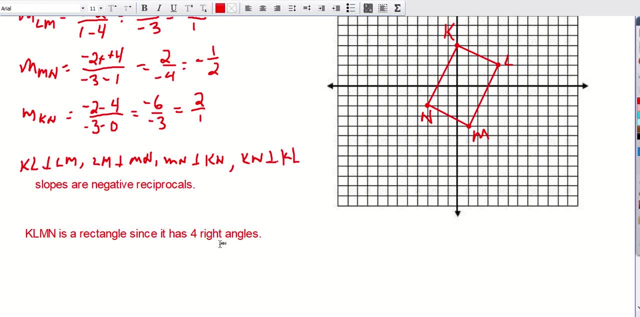 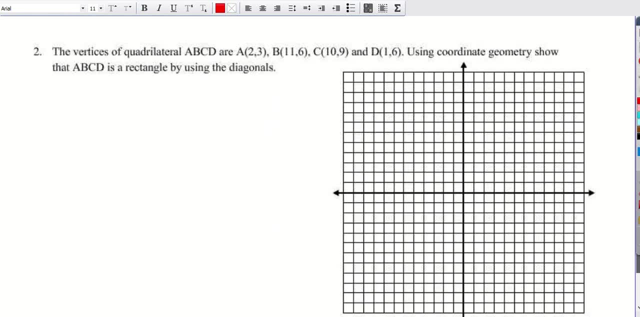 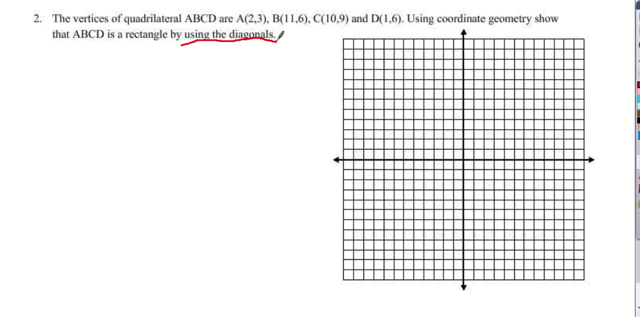 way to say that this is what's going on for my work and this is what's going on with the shape. All right, Number two: same thing. We're going to do: rectangle. This time we're going to use the diagonals. okay, If we're using the diagonals, we have to do two things. We have to say that it 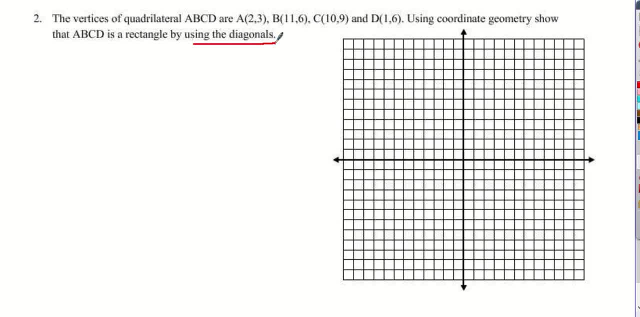 is a parallelogram first, and then we have to get it to be a rectangle, okay, So we got to do two things here. So we're going to go ahead and graph. So we're going to do a parallelogram first. 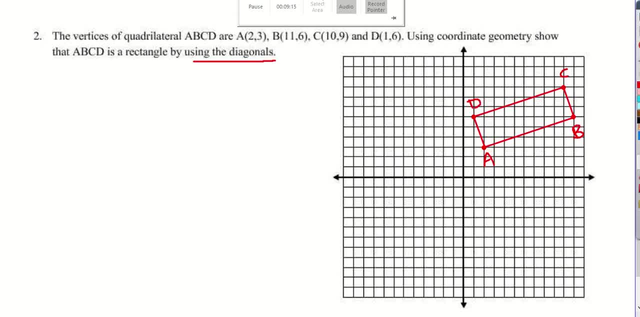 can grab first, All right, So we went ahead and we graphed, So now we have to use the diagonal. So two things we have to do is we have to get parallelogram first, Okay, And that's going to have the same midpoints, And then we have to say: so we're going to have 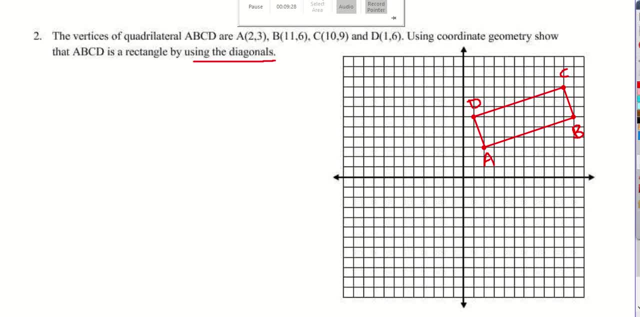 to use the midpoint formula to show that they bisect, And then we're going to have to use the distance formula to show that they're congruent. Okay, So for number one we're going to do that the midpoints are the same, So the diagonals bisect each other. So we're 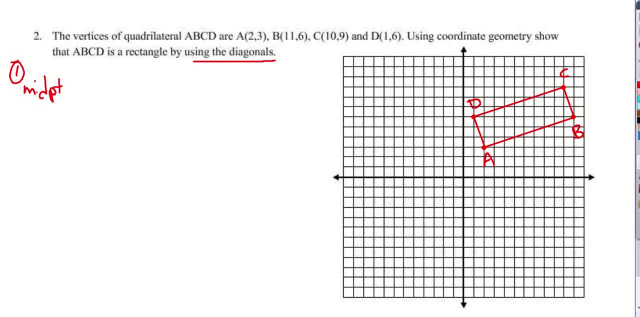 going to do the midpoint Okay, And we know we're going to look at the diagonals here, So we're going to do AC first. So remember, the midpoint formula is we add them and divide by two, So it's X2 plus X1 over two, and then Y2 plus Y1 over two, So this turns into so. 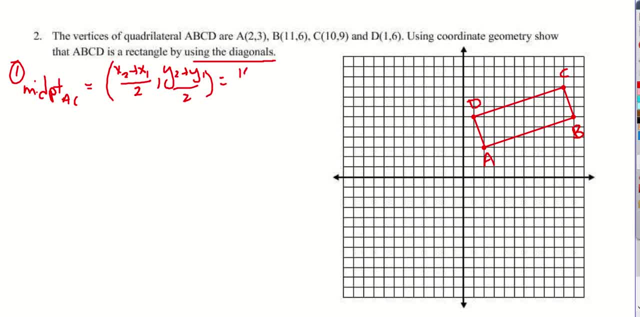 for AC, we're going to go to X2, which is 10 plus X1,, which is two over two Comma, and then nine for C plus A, which is three over two. And so here we're going to get the point 12, 12, or sorry, 12 over two, 12 over two until we get six, six as our. 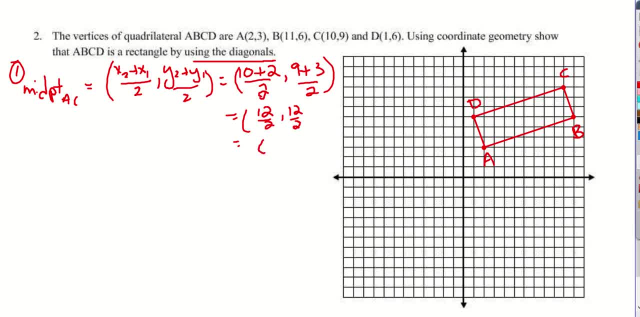 midpoint, And I am just trying to make these numbers legible. All right, And so this is the midpoint of AC. All right, And so the next one we're going to do is do DB. So midpoint of DB. I'm going. 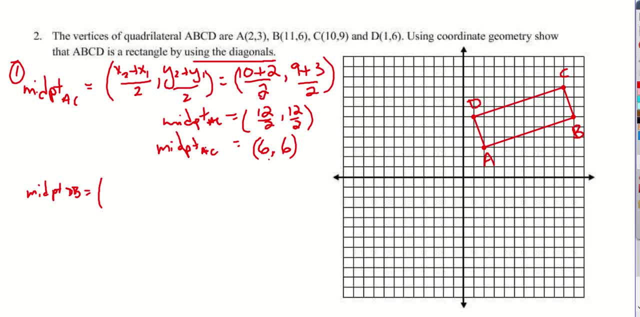 to go ahead and just plug the numbers in. So we're going to go to D first, So one plus B, All right. So we're going to do DB, which is 11 over two, and then six plus six over two, And so this is equal to 12 over two, 12 over two, And this is also equal to six. 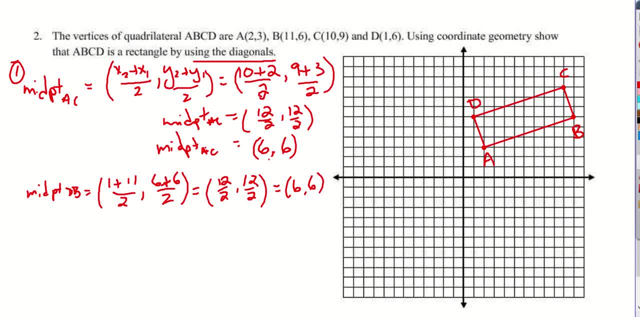 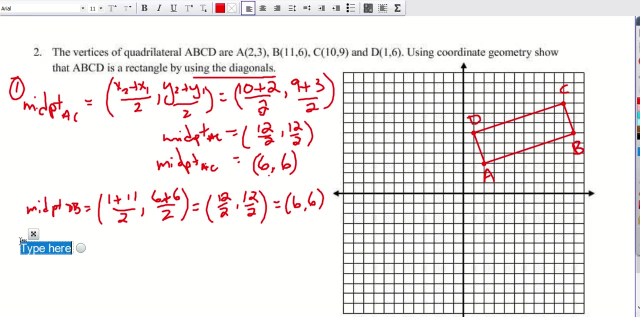 six, All right. So we're going to make a statement here. All right, We're going to say AC and DB bisect each other. I'm going to go ahead and type: Okay, So AC and DB bisect each other. 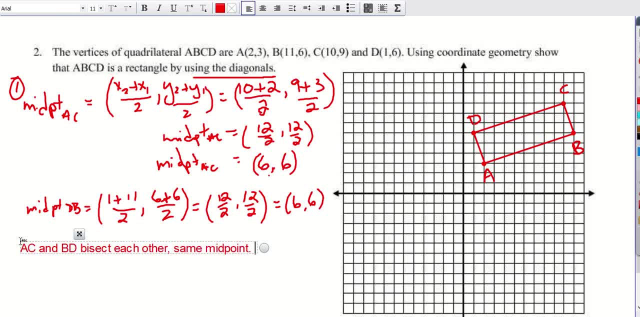 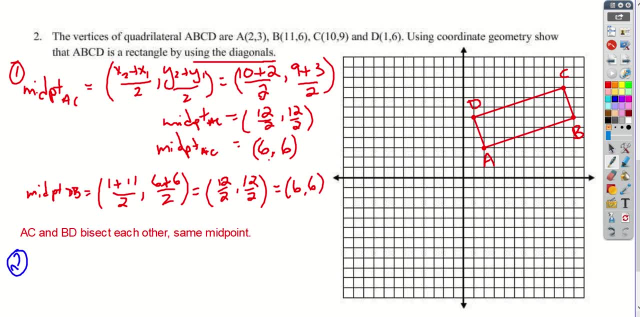 We know that because they have the same midpoint. All right, The next thing we're going to do is we're going to do the distance. So this is the second step. So we're going to do the distance of the diagonal. So that's AC. We're going to use the distance formula and then we'll. 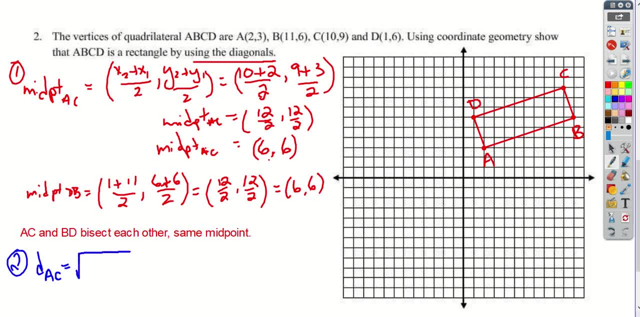 use Pythagorean theorem here. Okay, So the distance formula, if you remember, is X2 minus X1 squared, plus Y2 minus Y1 squared, And so this is equal to the square root of. So we're going AC, So X2 is 10 minus X1,. 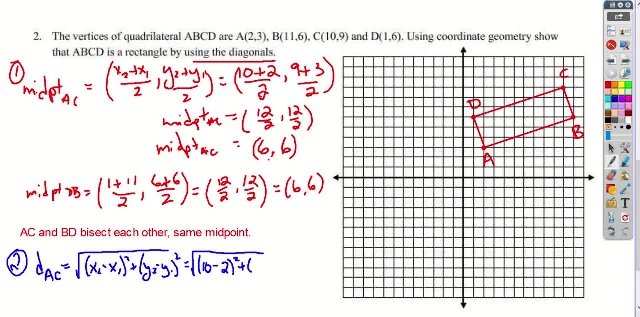 which is 2 squared plus Y2, which, for C, is going to be 9 minus 3 squared. Okay, And so this is equal to the square root of 8 squared plus 9 minus 3 is 6 squared, And so this essentially turns into: 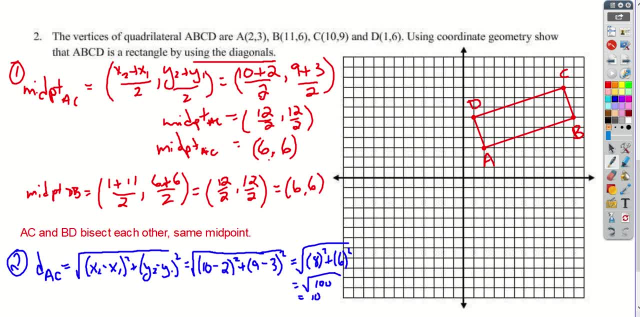 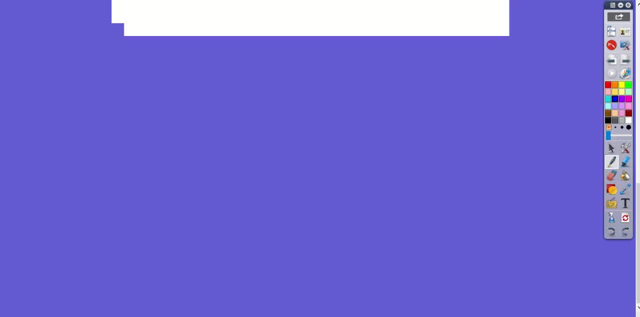 the square root of 100, which turns into 10.. Okay, So that's the distance of AC, And so we want DB to be the same distance. Okay, So I'm just going to shrink this down a little bit so I can see both here as we go We'll do 150.. See if that makes. 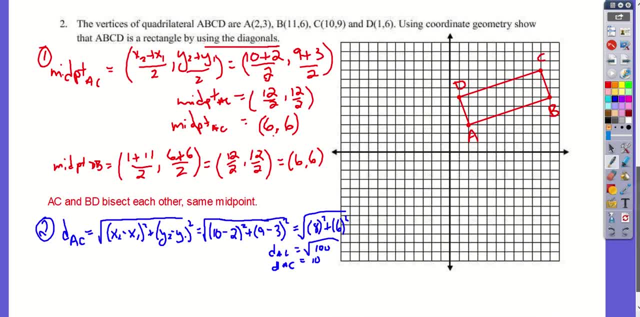 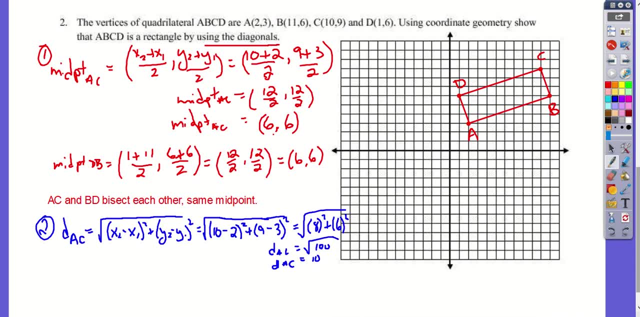 any better. I think it does All right. So the second we're going to do is we're going to do the distance of DB, Okay, And so we're going to do the distance of AC, And so we're going to do. 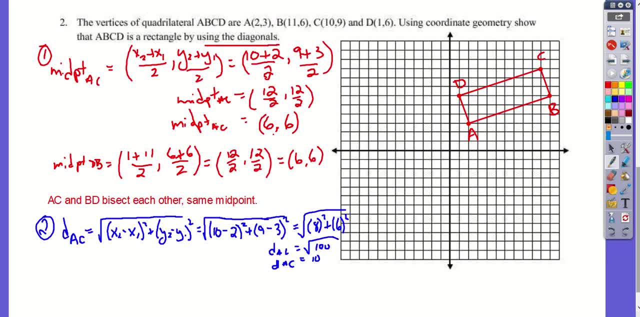 the distance of DB. So we're going to go ahead and mark. Actually, we don't have to mark, We can just count straight across. Look at that Right: 1, 2,, 3,, 4,, 5,, 6,, 7,, 8,, 9,, 10.. We don't even have. 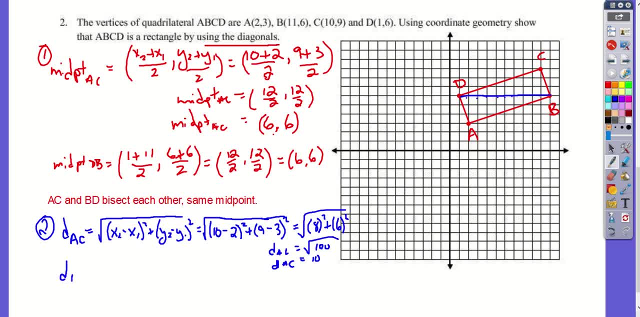 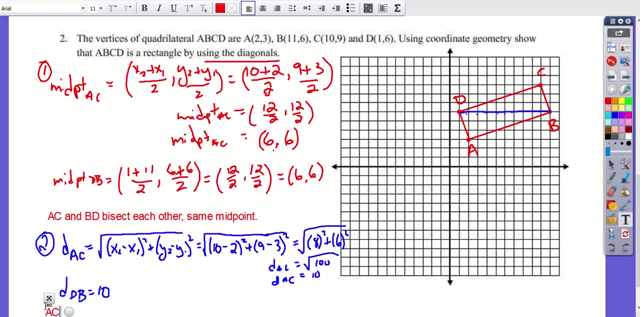 to show any work, We can just do D and then it's DB equals 10.. Okay, That's it. And so now we're going to write our second statement and then our summary statement. So we're going to say: AC is equal or congruent. Let's use congruent, Proper math terminology here. DB, since the